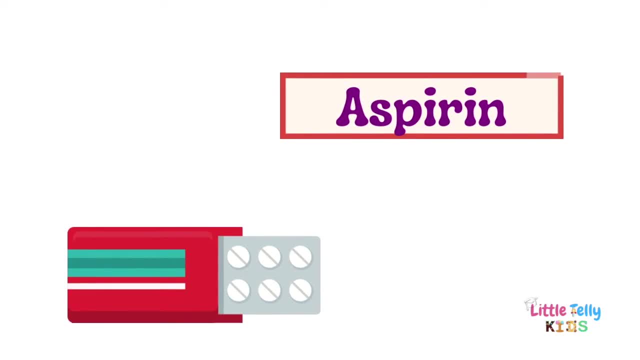 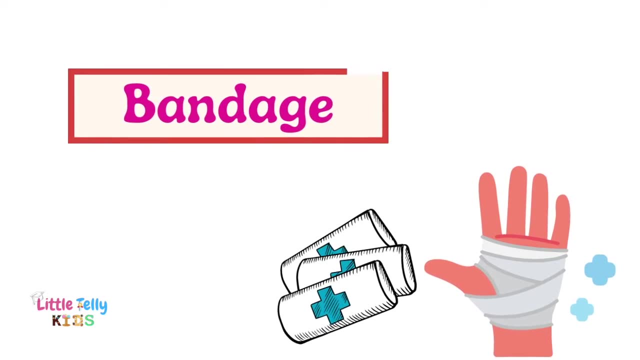 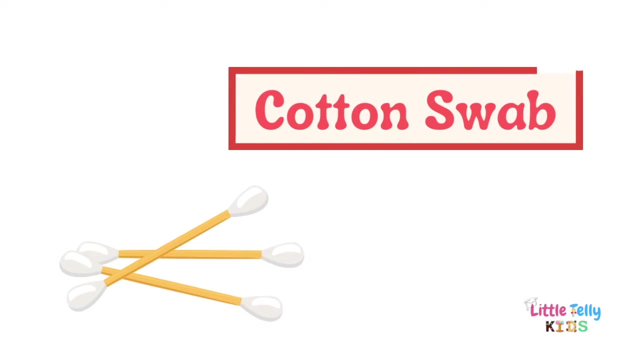 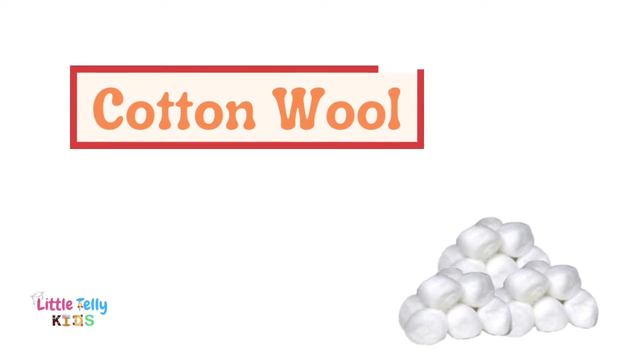 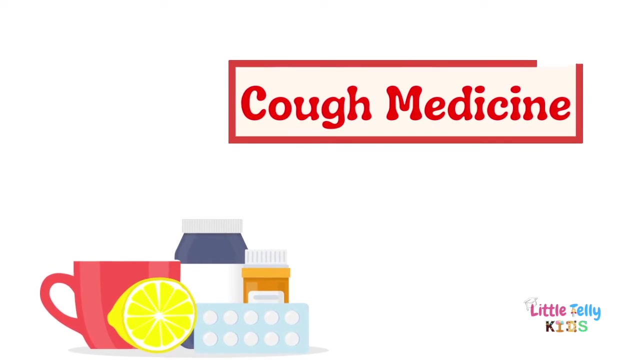 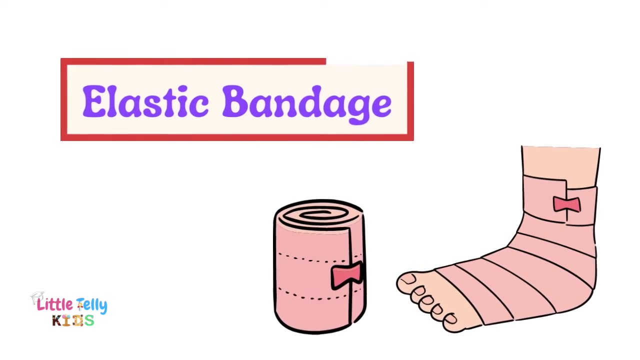 Aspirin. Aspirin Bandage. Bandage Cotton. swab Cotton. swab Subscribe. Cotton. wool Cotton. wool Cough medicine. Cough medicine. Elastic bandage. Elastic bandage. First aid kit. First aid kit. 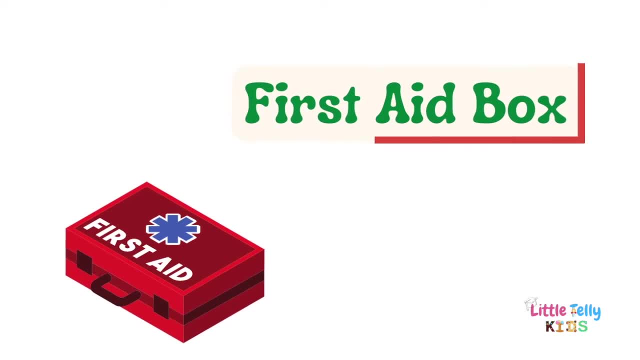 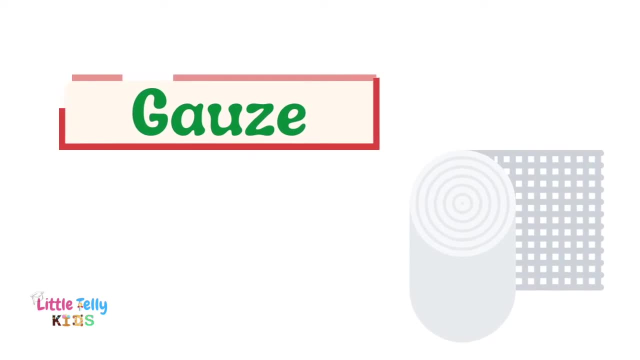 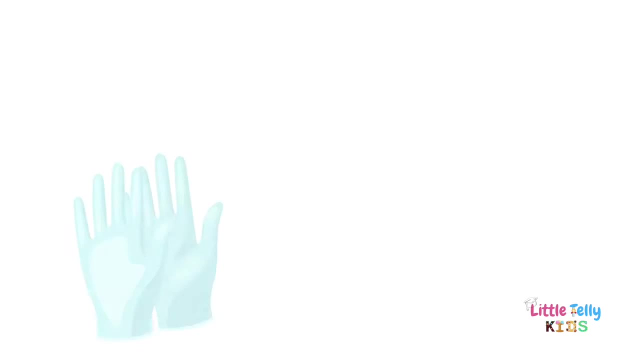 First aid box. First aid box, Gauze Gauze, Gloves, Gloves, Medical wipes, Medical wipes, Net bandage, Net bandage, Pain killers, Pain killers, Plaster, Plaster, Pyridine, Pyridine. 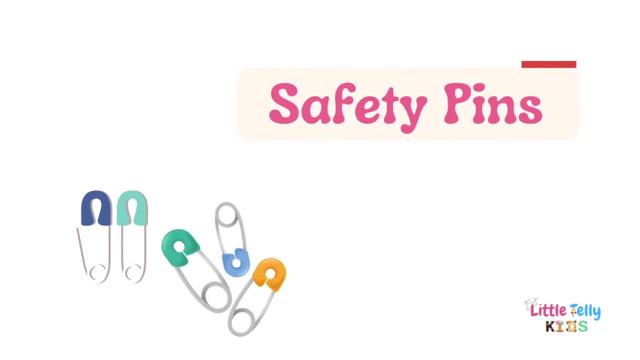 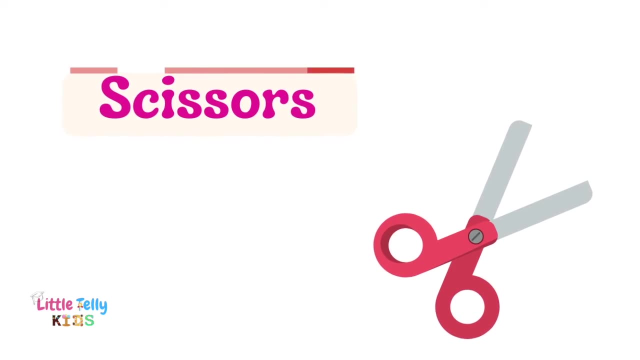 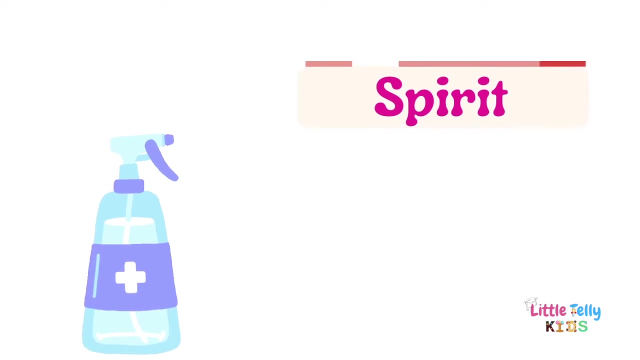 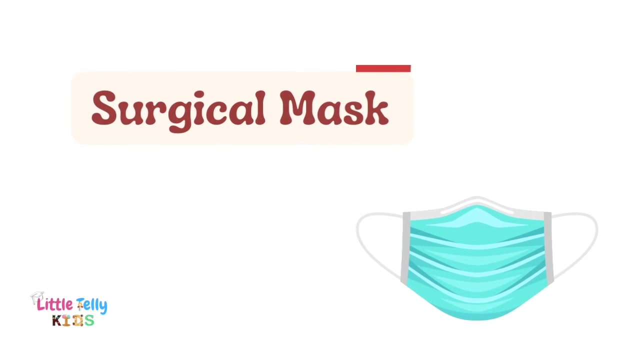 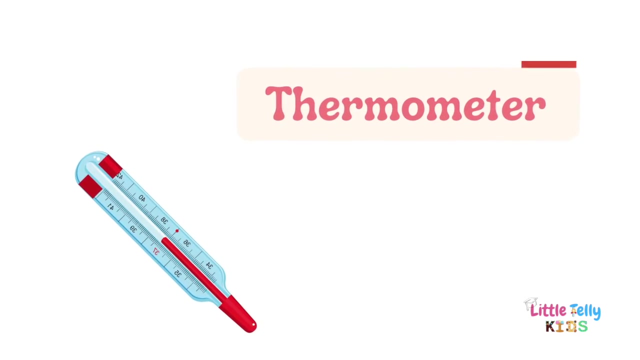 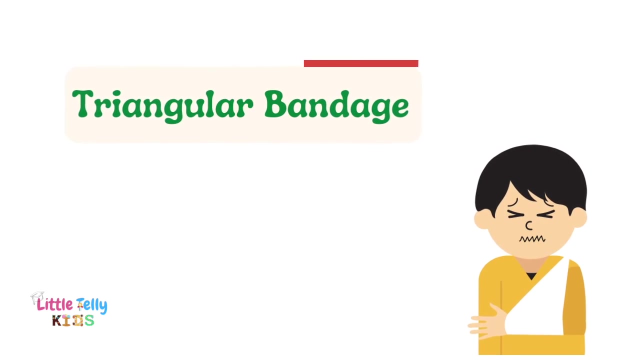 Safety pins, Safety pins, Safety pins: Scissors, Scissors, Scissors, Like Spirit, Spirit. Surgical mask, Surgical mask, Thermometer, Thermometer, Thermometer Thermometer. Triangular bandage. Triangular bandage. 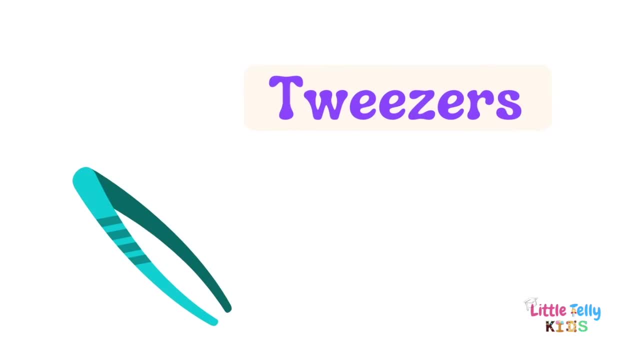 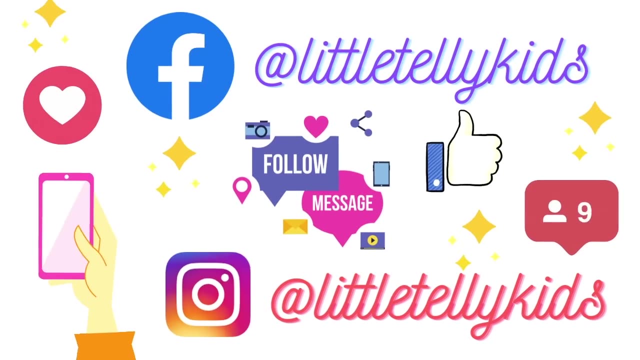 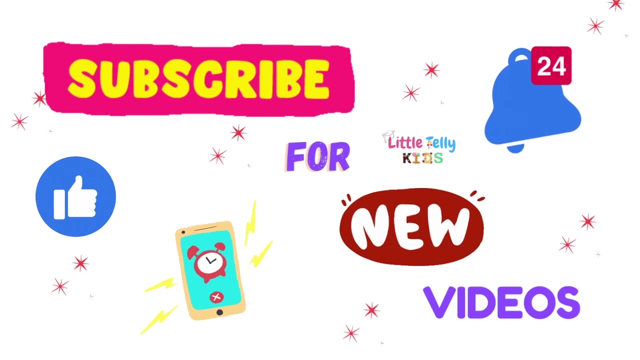